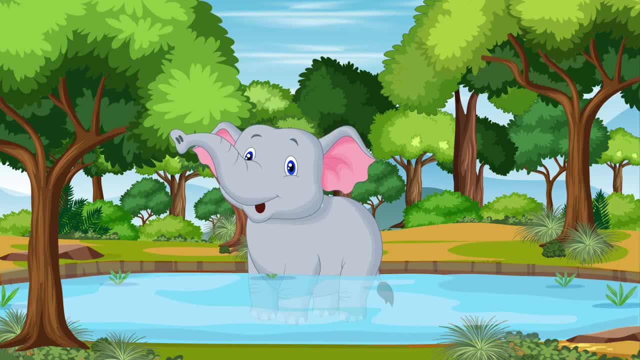 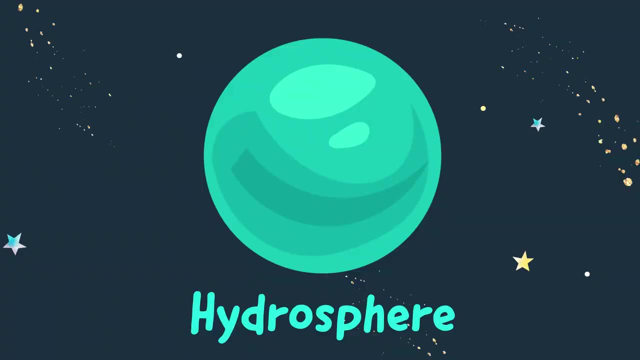 stay nice and warm, Sometimes a little too warm, which leads me to the hydrosphere. The hydrosphere contains all of the water on earth in liquid, solid and vapor form- About 71% of the earth's surface. 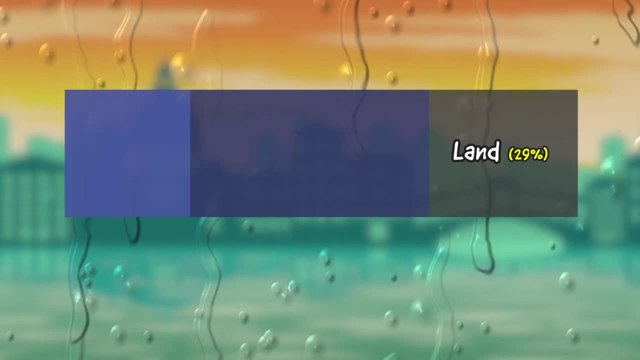 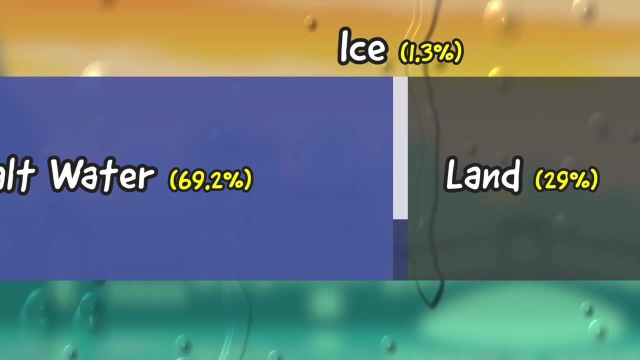 is covered in water, but nearly all of that is saltwater in the oceans and the seas. Most of the freshwater that does exist is frozen in the polar ice caps, glaciers and icebergs, with only a small amount of liquid water in the lake. 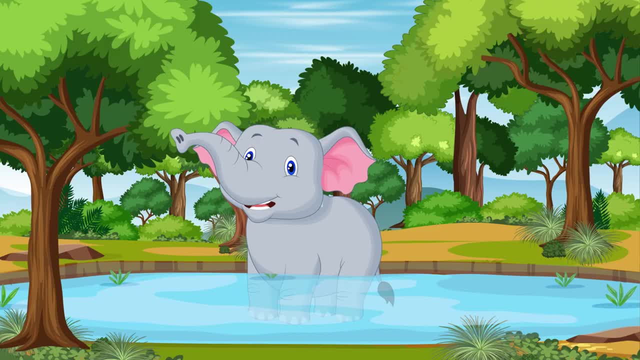 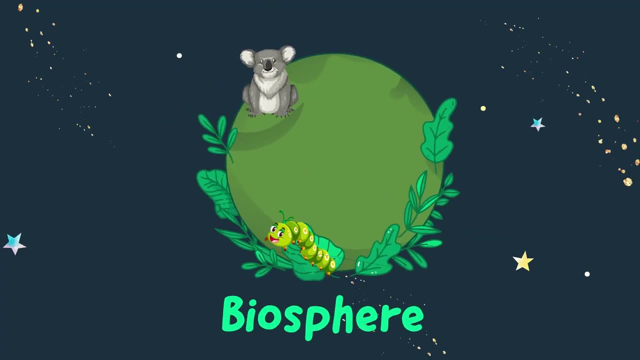 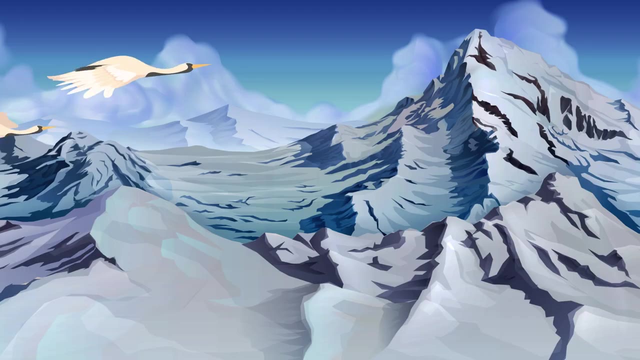 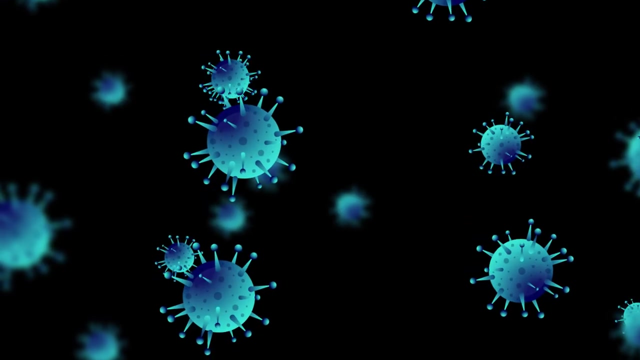 I'm going to show you how that works. And finally, the biosphere makes up all of the living things on earth. Life exists all over the earth, from the darkest depths of the ocean to the skies above the tallest mountains. Plants, animals like me, humans, and even tiny bacteria and viruses are all. 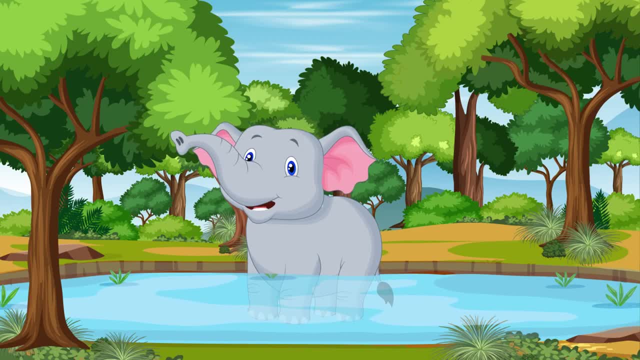 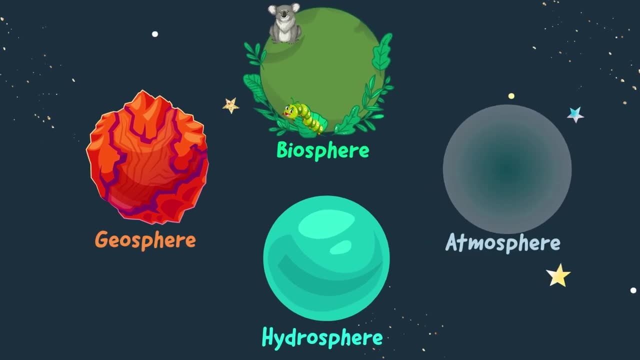 part of the biosphere. And those are the four spheres. Okay, time for a swim. Thanks, Eli, Have fun. Okay, let's see how each sphere interacts with the others, starting with the hydrosphere and the geosphere. 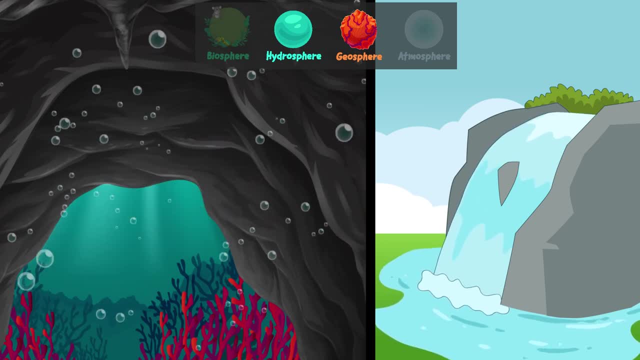 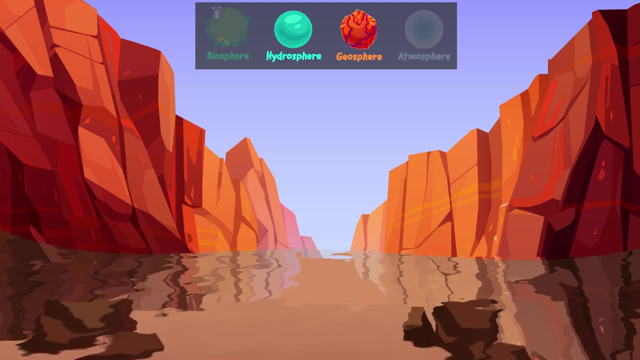 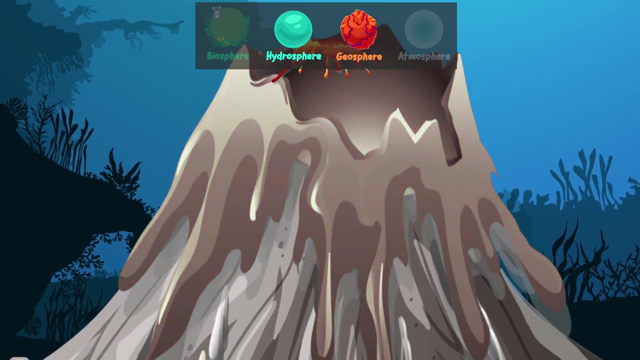 Water shapes the geosphere through erosion and creates features like caves and waterfalls. One of the best known examples of water erosion is the Grand Canyon, a mile-deep gorge carved by the Colorado River over millions of years. When large volcanoes erupt underwater, the 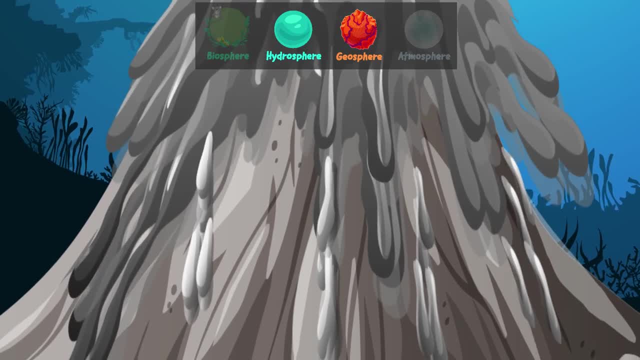 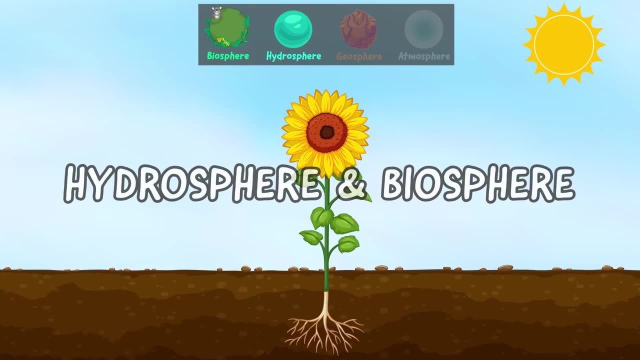 water cools the lava, And water in the ocean is the very source of oxygen that is made lava and solidifies it. The lava rock builds up over time and sometimes emerges out of the water to form islands. Living beings in the biosphere need the hydrosphere to live. 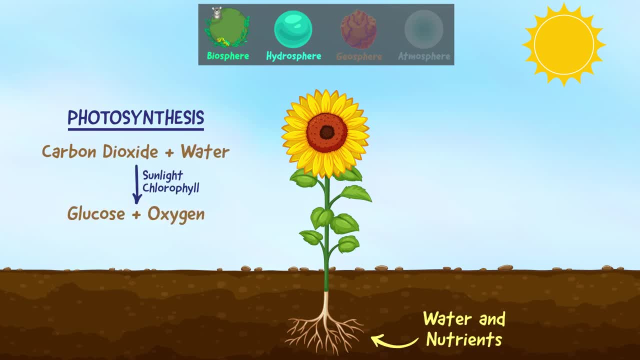 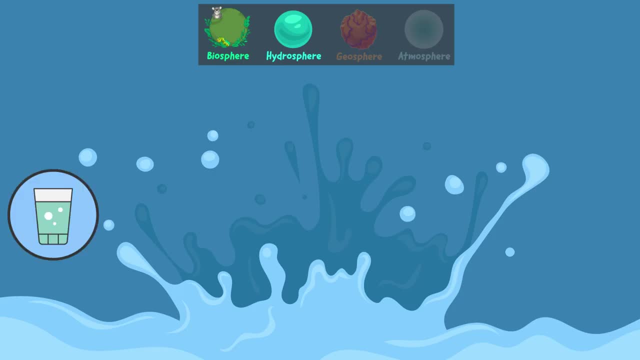 Plant roots absorb water for photosynthesis to create energy, and the water also helps transfer nutrients from the soil to the plants. Animals like Ellie need water to live. Humans use water for not just drinking but also cleaning, farming, cooking in industry and 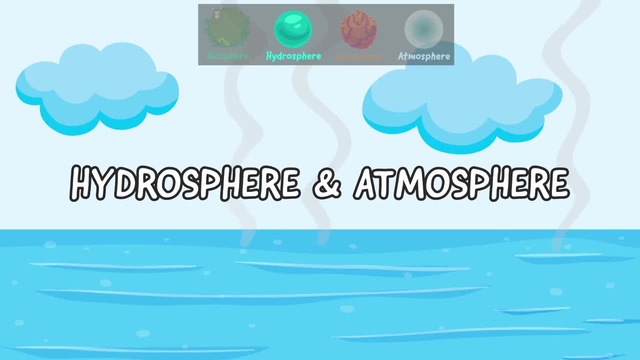 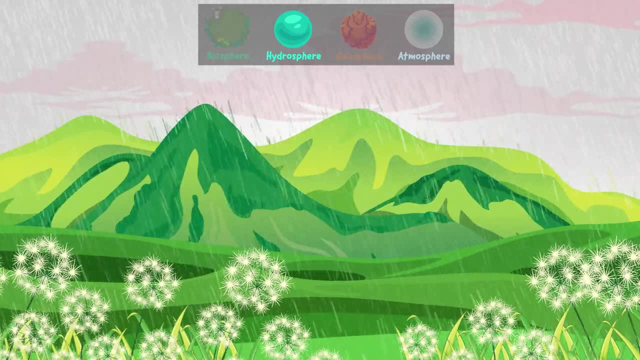 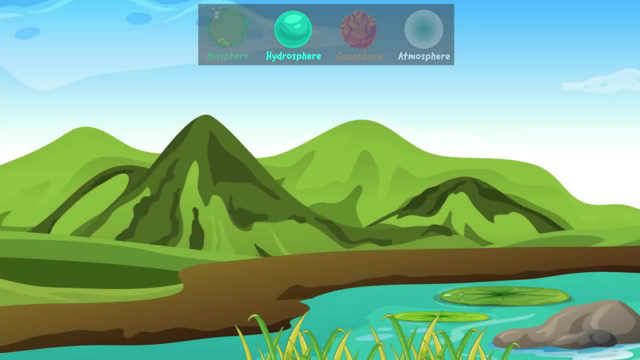 many other uses. Water, mostly from oceans, evaporates into the atmosphere as water vapor, then condenses to form clouds and then falls back to the earth as rain or snow. Snow melts into rivers and rivers flow back into oceans. This constant cycle shapes our climate. transports.